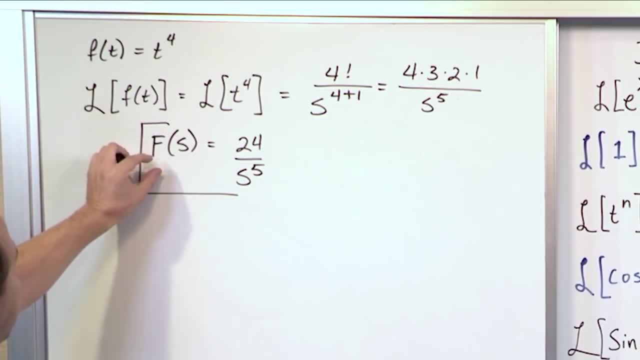 say function of time, function of s, The f goes with the big F. That just lets you know that these are linked by this transform. We use that sort of symbology there, But really it's its own independent function of s which is really the Laplace Transform of f. And 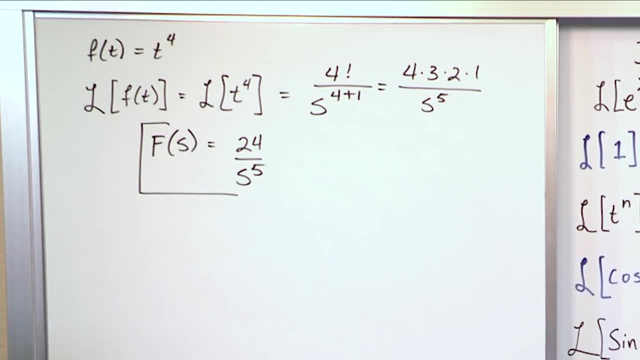 so what we're going to do is we're going to take this function of s, which is representing the function, but in the Laplace domain or in the s domain. All right now the next problem- Let me switch colors- What if we have f of t is sine of 2 times t, And you want to find: 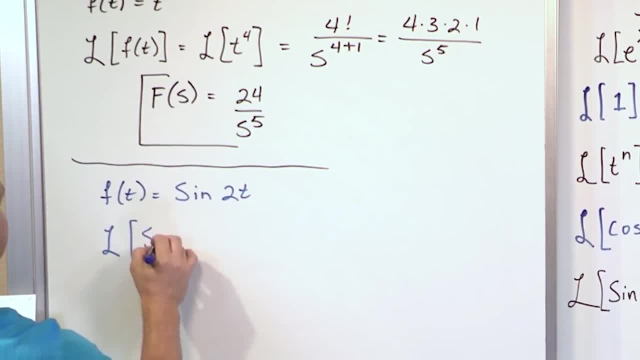 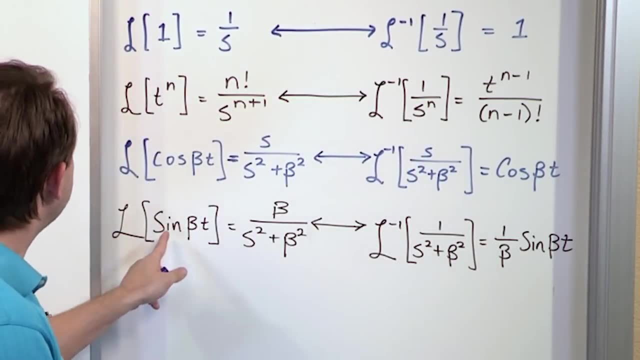 the Laplace Transform of this, So say Laplace Transform of sine 2t, And you go over here and say, is there anything that looks like that? And of course we have a sine function right here. In this case beta would be 2.. Sine 2t, beta would be 2.. It's going to be beta over s? squared. 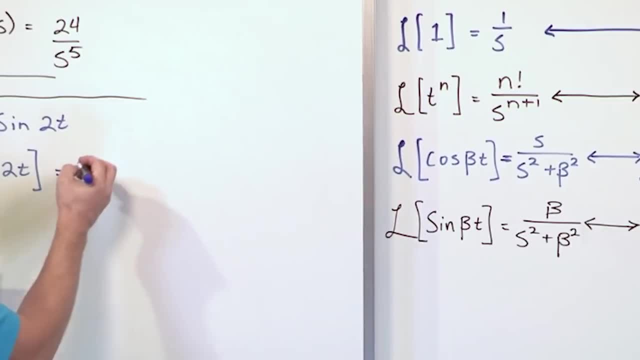 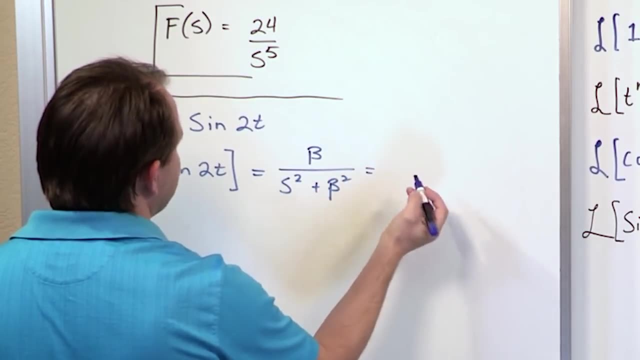 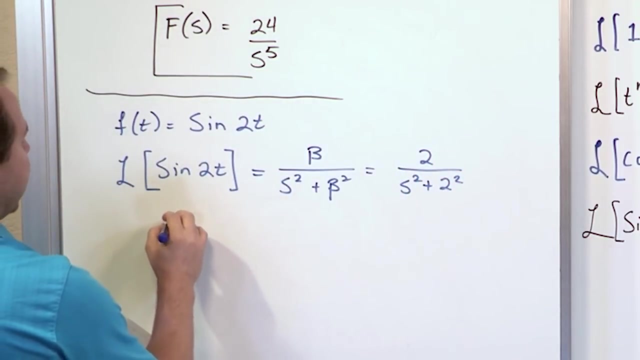 plus beta squared. Here beta is equal to 2.. So you can just refresh my memory at beta over s squared plus beta squared, where beta is equal to 2.. So it's going to be 2 over s squared plus 2 squared, And so to write the full answer, you can say: f is a function. 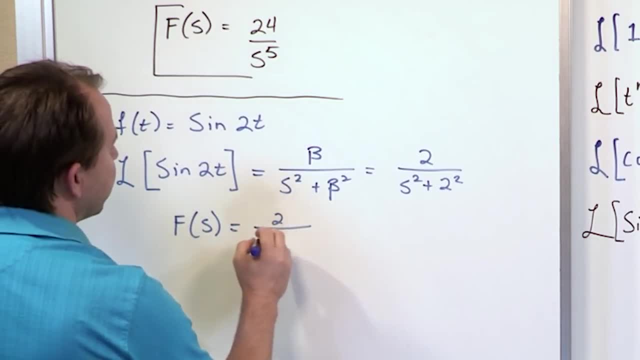 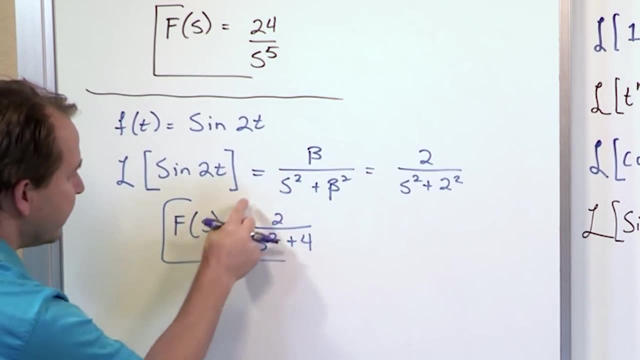 of s, which implies that you've already transformed it. It's 2 over s squared plus 2.. So you're going to have 4.. And that's what you would circle again on your exam. So notice, you have a function of s. There's nothing else here except s's. All right, we've. 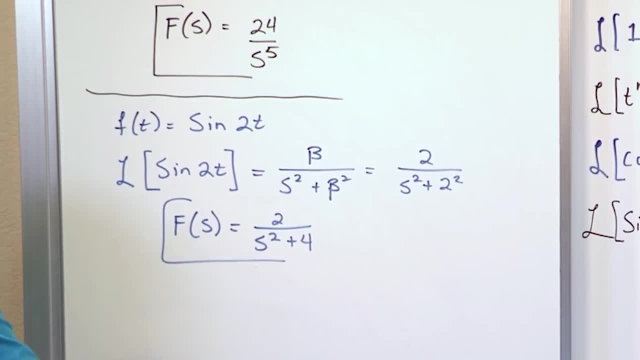 locked down this value of beta when I was given this specific problem at hand. All right, so let me go ahead and erase the board here And we'll work on our next couple of problems, which are really no harder, but we're just going to work our way through our skills. 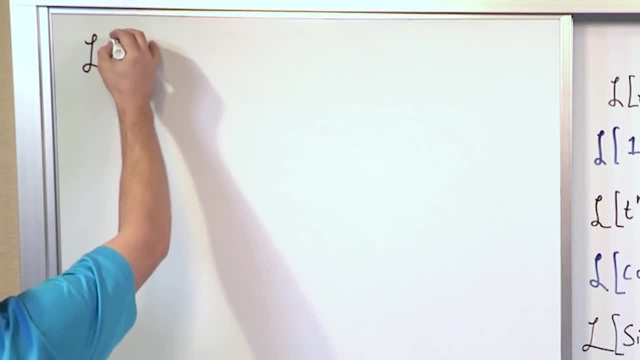 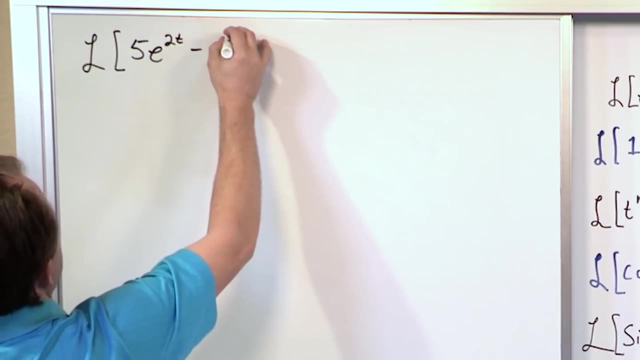 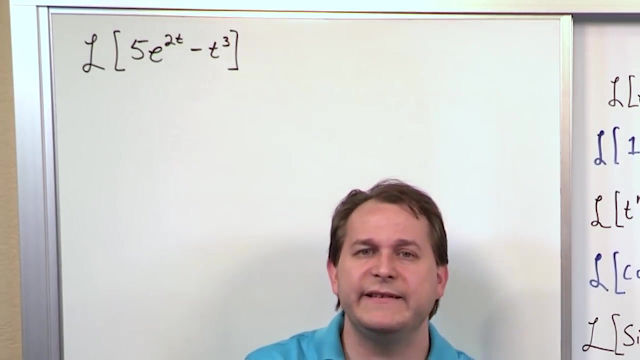 All right. now the next problem says: let's take the Laplace Transform of 5 times e to the 2t minus t cubed And, furthermore, let's try to write it out in integral form, not because we want to do all the calculus, but just to see how it would look, because that 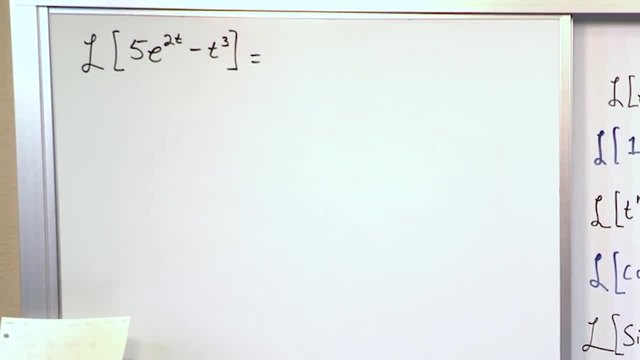 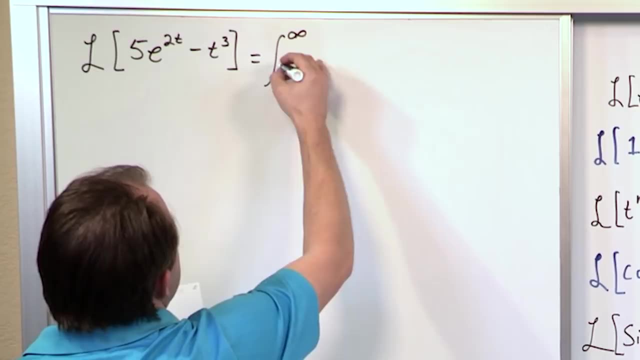 can definitely give you some experience too. All right, so what you would have if you were doing it by the definition of the transform, which we're just doing here for clarity, just to kind of show you integral e to the minus st, And then you open up parentheses and dump: 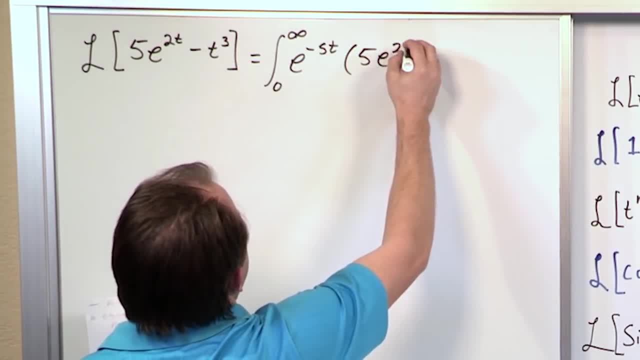 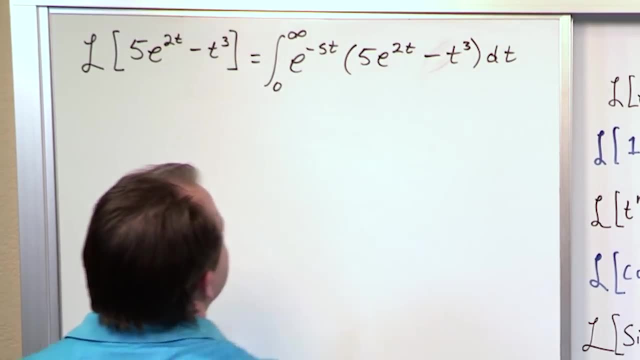 your function. And your function is a linear combination of two things: It's got an exponential and it's got a minus sign here, actually, And it's got t cubed dt. So if I didn't know anything about this table of transforms, I would dump this in and I would try to integrate it. 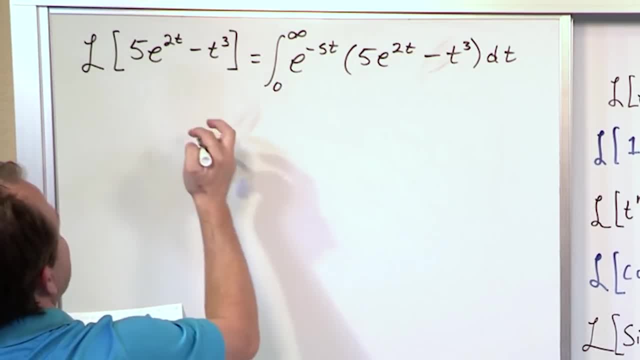 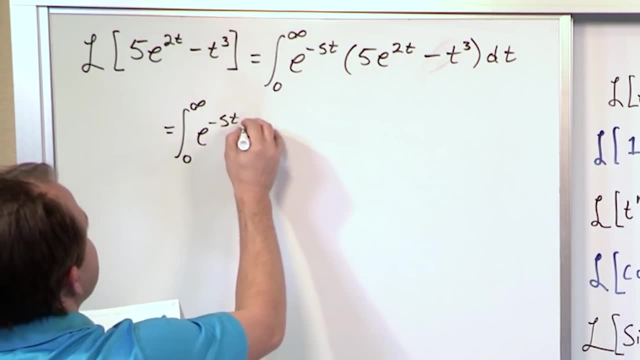 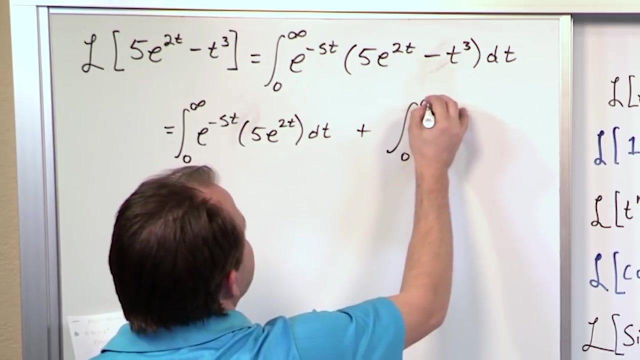 And furthermore I can rewrite this. Let me go to the left a little bit. I can rewrite this as integral 0 to infinity e to the minus st 5e to the 2t dt. And then I can write this as integral 0 to infinity e to the minus st negative t, cubed dt. Make sure you understand. 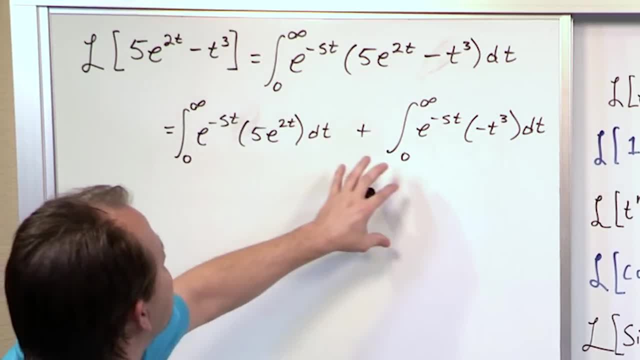 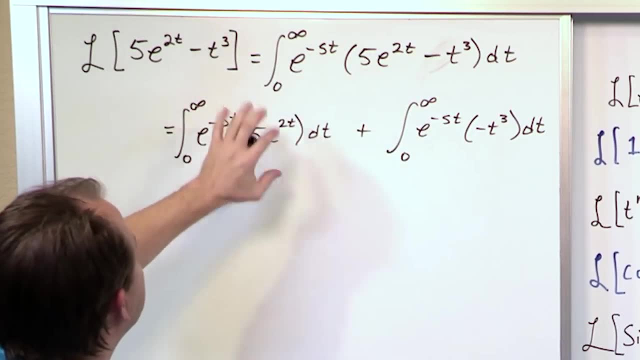 this. All I'm doing is I'm saying, look, I can break this integral up into two pieces And I can say, because what I can do is I can take this exponential and multiply it in times, this, That's going to be one integral. I can also multiply it in by this, This negative. 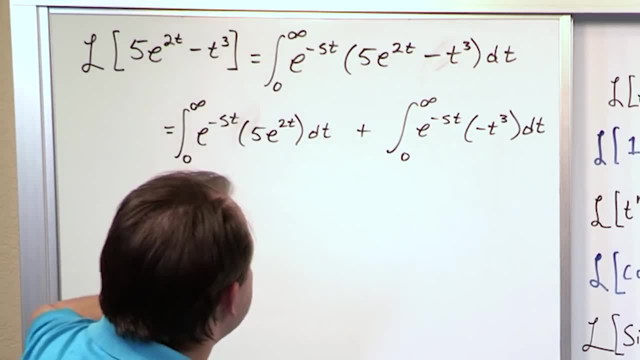 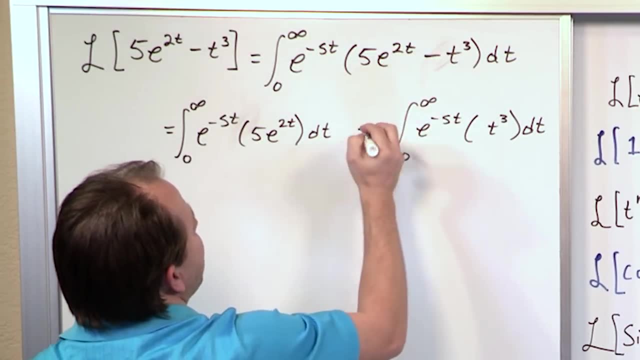 I'm keeping track of here, And so that becomes a positive. And so basically, I have two guys right there And if I want to, since it's just a constant, I can take that negative and I can pull it out. It's the same exact thing. So what I've done here is I've shown you from calculus. 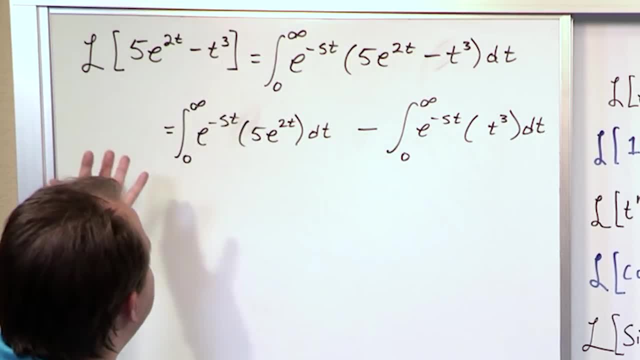 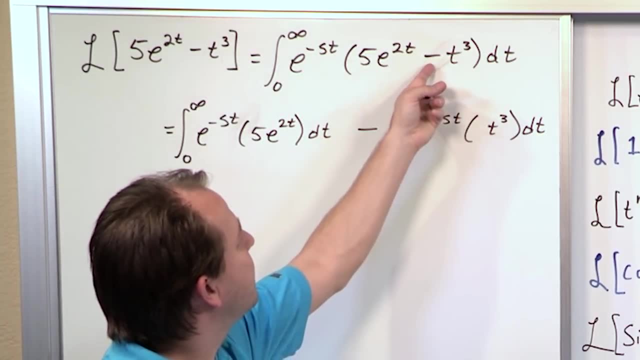 because it's just an integral, that because you have a linear combination of two things, it's basically applying the Laplace transform separately, Once to this guy and then secondly to this guy. Any pluses or minus just basically link the two guys together. So another way. 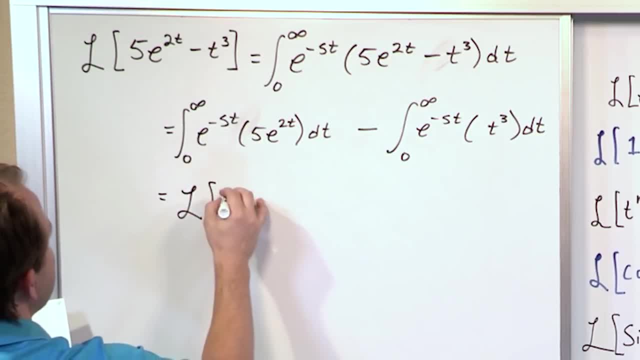 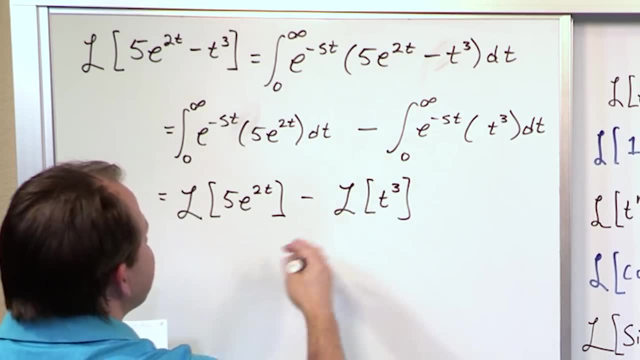 to write. this is Laplace transform of 5e to the 2t dt, Minus Laplace transform t cubed. So this is kind of what your first instinct would have been anyway If I had given you this problem and I said: what's the Laplace transform? 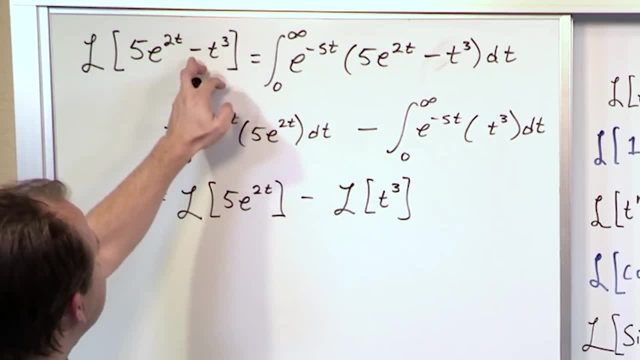 You apply it to the first term, You apply it to the second term. Whatever is here plus minus just links them together. I'm just going through the integral here to kind of show you that by calculus that basically it all connects together and it works. So that's. 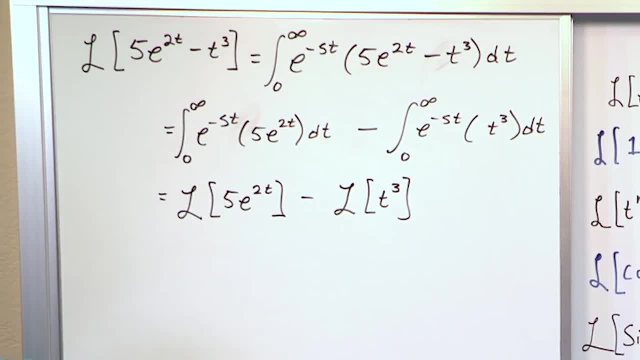 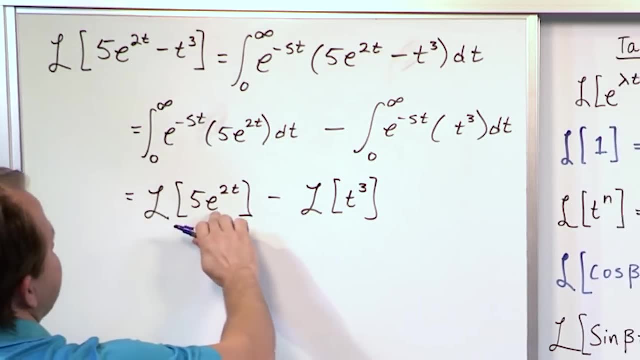 linearity. That's the property we discussed. Now that we got down to this level, we can apply the transform separately. Let's go ahead and do it All right. So does anything look like this? e to the 2t. Well, we see right here. e to 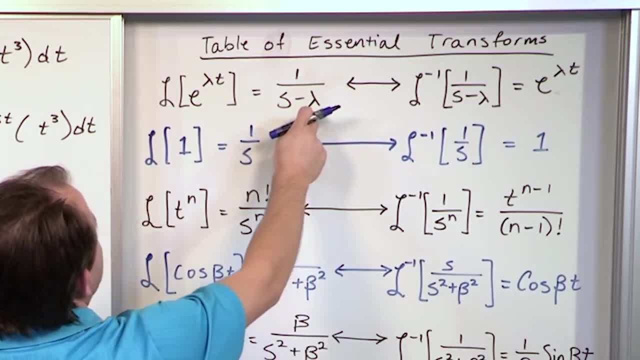 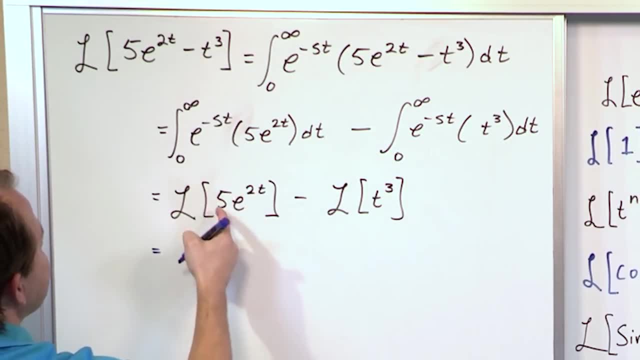 the 2t fits this. 1 over s minus 2 is what it would be there, But we have this 5 out front. But don't forget, we actually said when we talked about linearity that any constants in the function can be pulled out, Because, just as you see here, it's just an integral. 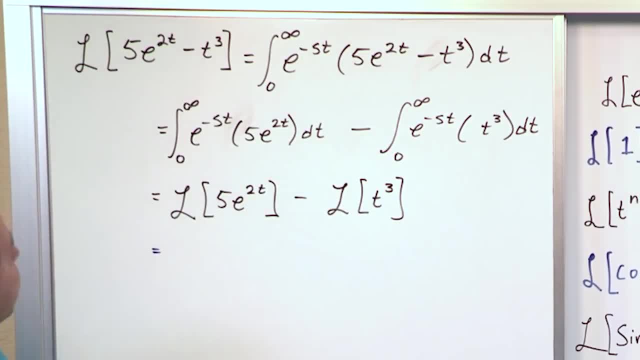 So the constants can come out. here There's really only a 1 that comes out, So there's nothing to show there. So what it becomes then is it becomes 5.. 5 times the Laplace transform of this, which we already said, is 1 over s minus 2.. That's. 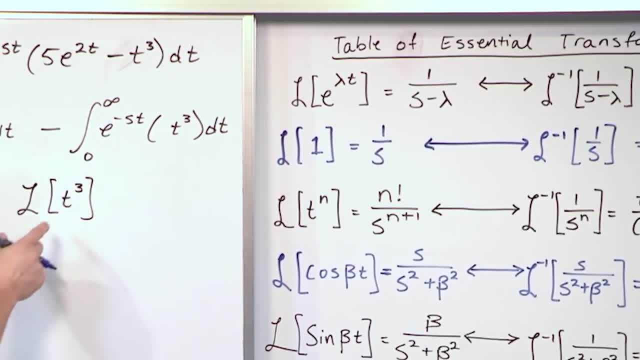 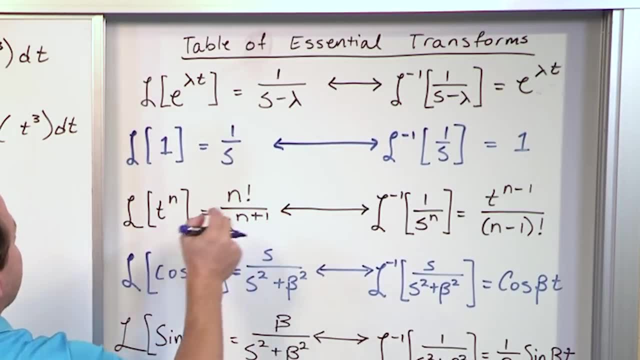 the Laplace transform of e to the 2t. Then we subtract off. We say what's the Laplace transform of t cubed? We go here, We say that it's going to be 3 factorial s to the m plus. 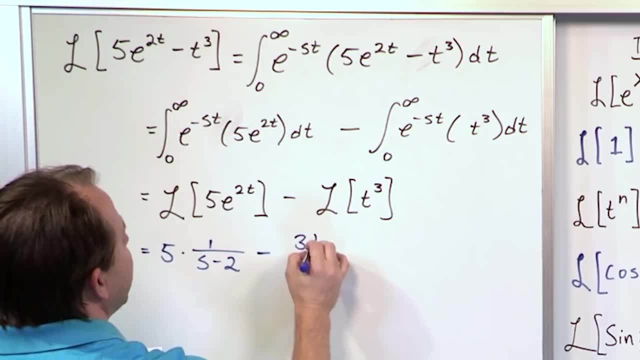 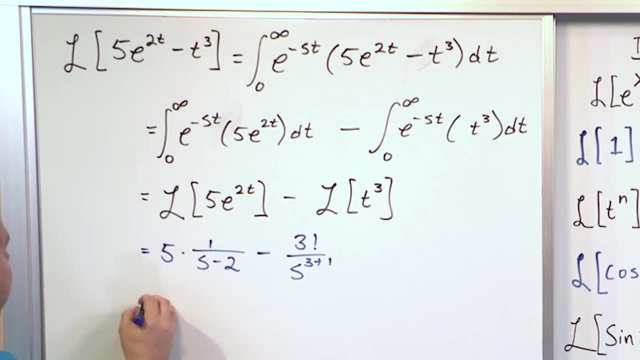 1, which would be s to the fourth power. So we say, just to show it, we say 3 factorial s to the 3 plus 1.. I don't like to do too many things in one step, So I like to show. 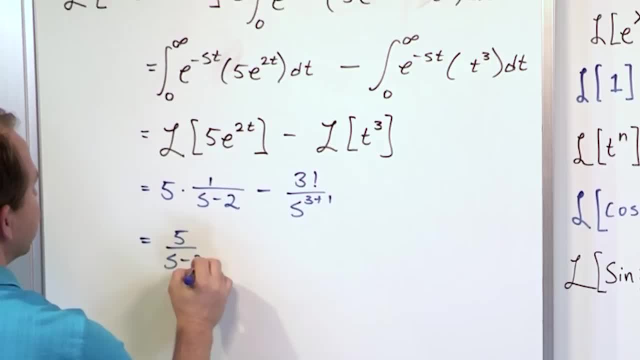 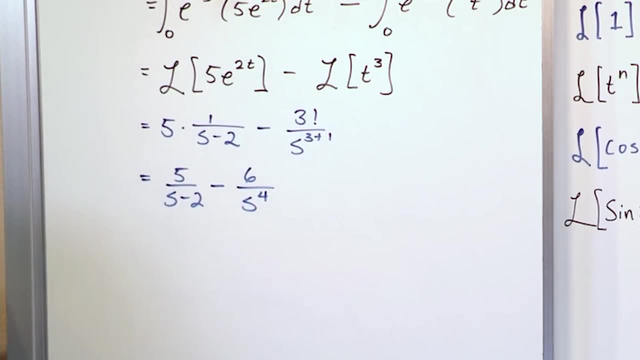 everything. So I get 5 over s minus 2. minus 3 times 2 is 6 times 1 is still 6 over s to the fourth power. So I get 5 over s minus 2 minus 6 over s to the fourth. This is f capital of s, because 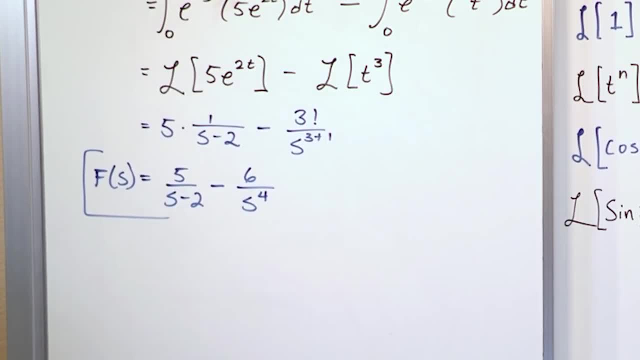 it's a function of, it's a pure function of s. So notice that what's happening Every time we transform these guys is: I go from a function of t to a pure function of s. It gets confusing whenever you first learn about the transform. 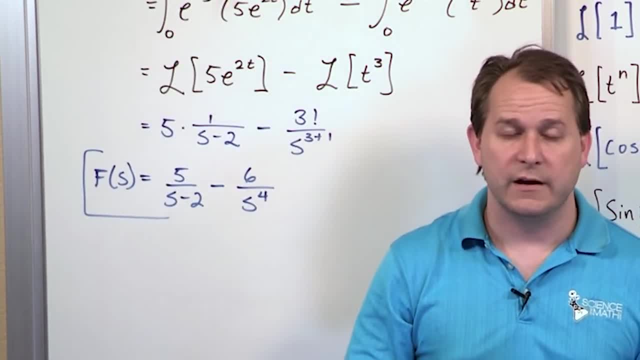 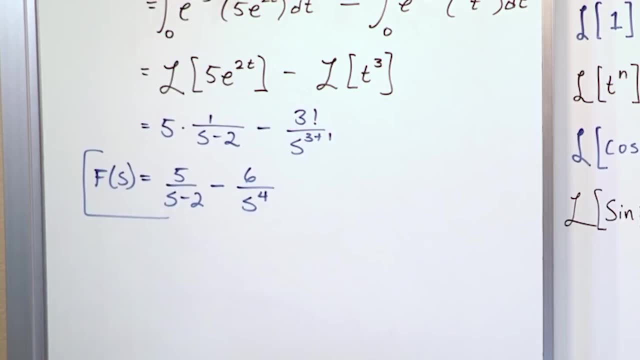 the thetas and lambdas and stuff running around, But those are just constants. Those are locked down by your problem. You should end up with a pure function of s. That's what the Laplace transform is All right. So let's go on to the final problem in this lesson, which is going to be what? 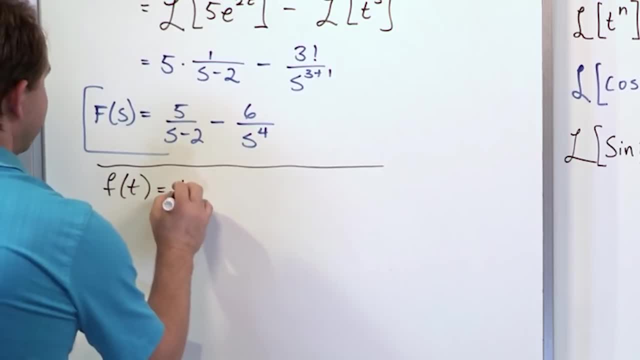 if I have the function f of t is t squared minus 7 plus cosine of 2t. How do we take the Laplace transform of this? So we say Laplace transform of f of t. So we say Laplace transform of f of t. 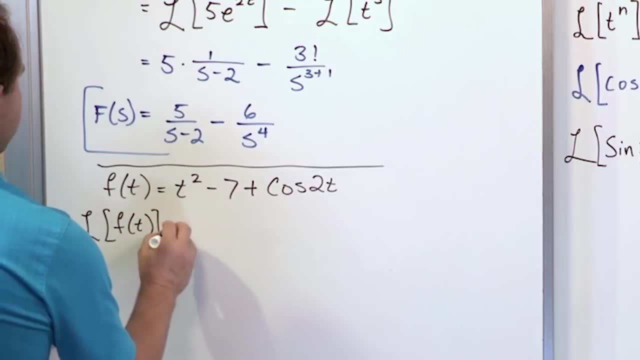 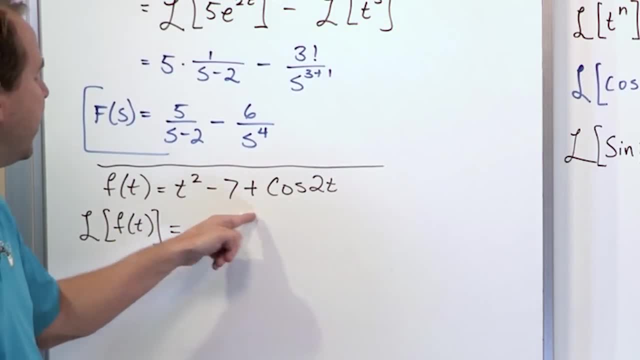 three terms. Here we have linked by a minus, Here we have linked by a plus. But from the linearity you should now know that we just apply the Laplace transform to each little piece separately, just like we do in integration. The minuses and pluses will just link the. 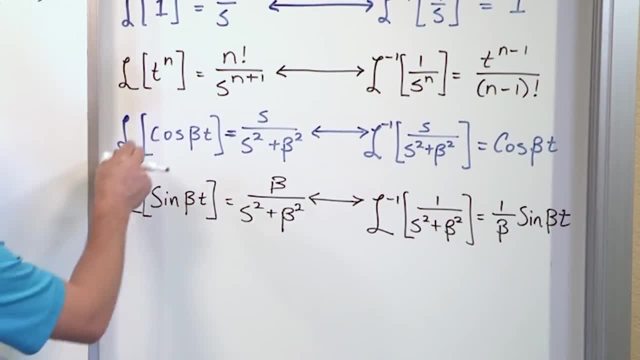 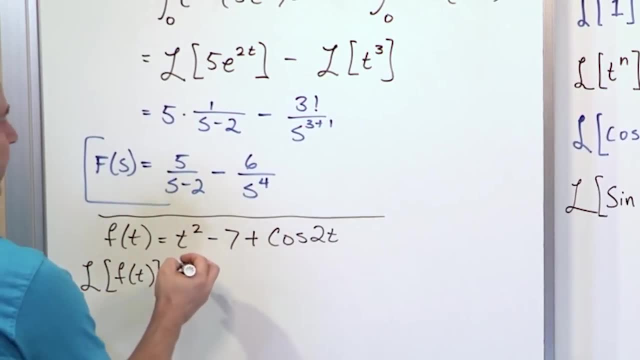 answer. So we go and look at t squared. T squared fits this mold, So it'll be two factorial over s to the 2 plus 1.. So what we're going to write here is 2 factorial over s to the 2, factorial over s to the 2 plus 1, that's going to be the first term, and then we carry. 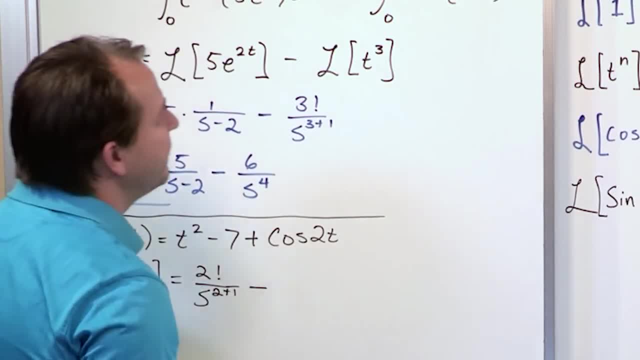 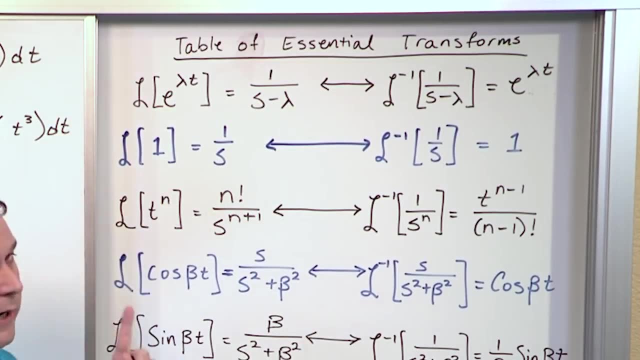 the minus sign, which comes from here, and then we have to take the Laplace transform of 7.. Now we don't have a Laplace transform of 7, okay, obviously we don't have that, but we have the Laplace transform of 1.. 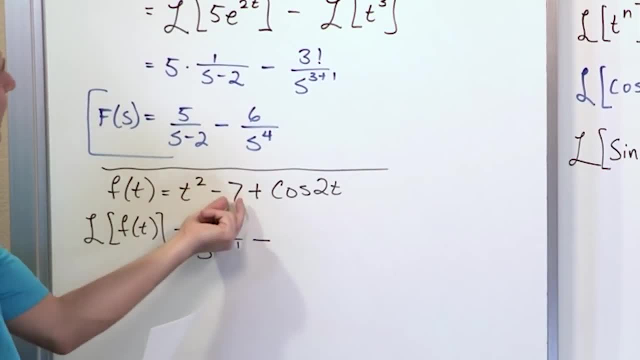 So notice that 7, right, is just a constant. You can write 7 as 7 times 1, right? So you can think of it as pulling the 7 outside, for lack of a better word. and now it's the. 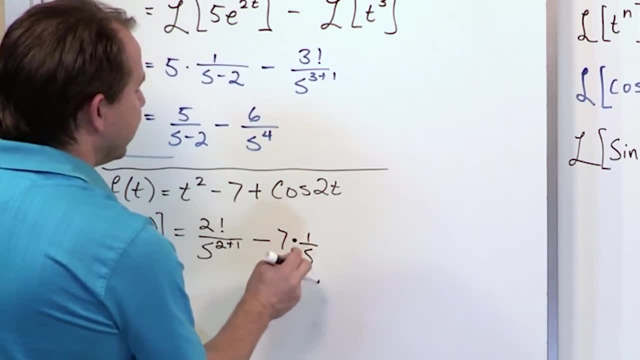 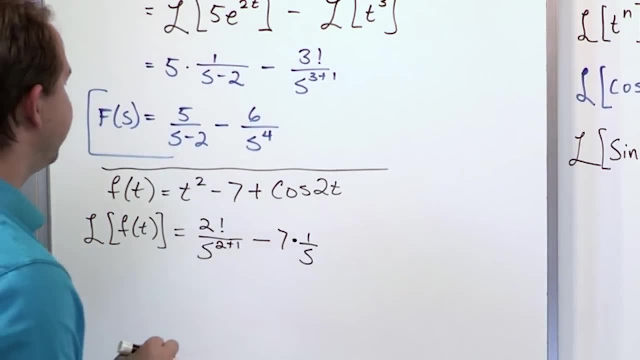 Laplace transform of 1, which is 1 over s. So 7 times 1, 7 is pulled out because it's a constant Laplace transform of 1 is 1 over s, And that's how you get this guy, and then the plus sign links it here, and now you have. 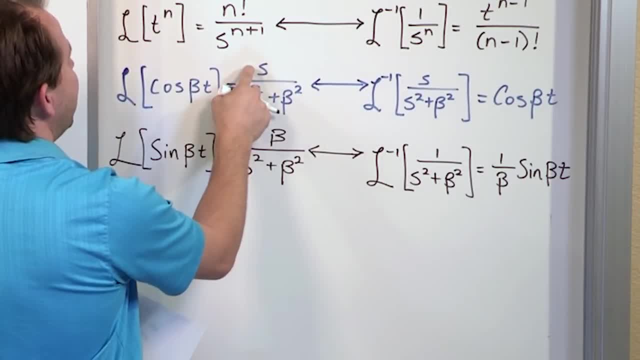 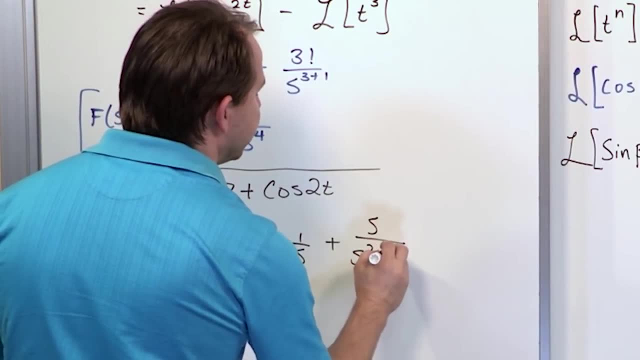 cosine 2t. so here's cosine. so you have s over s squared plus beta squared, so that's going to be 2 squared. So it's going to be s over s squared plus 2 squared, And so the final answer. 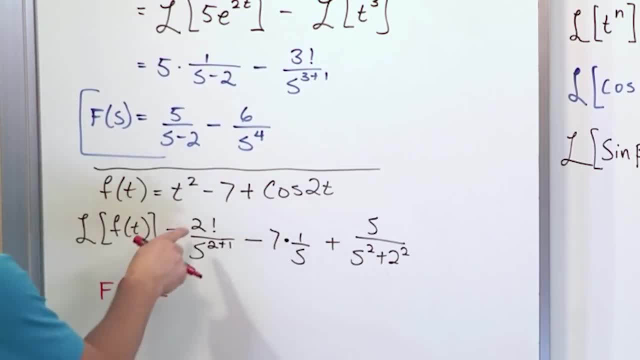 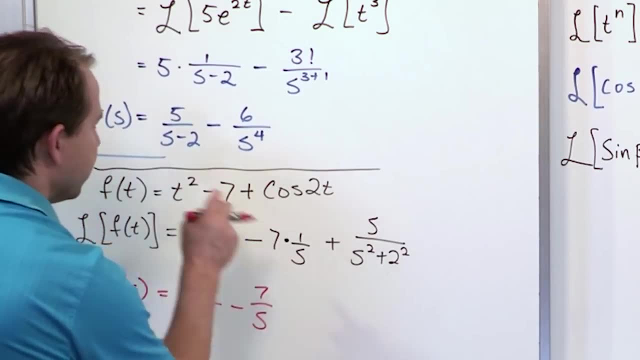 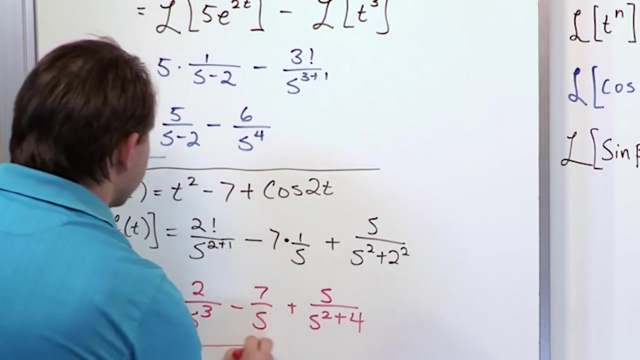 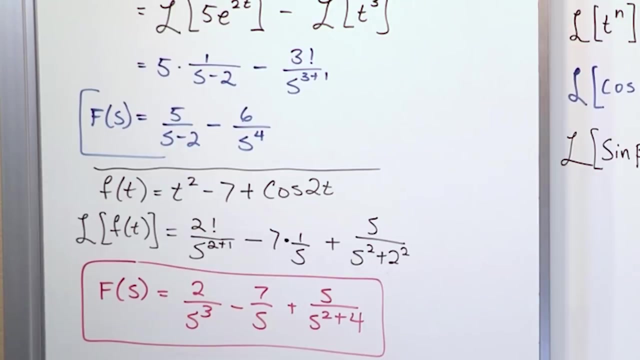 is f of s here. 2 factorial is just 2 s cubed is what you'll have on the bottom, minus 7 over s for the middle term, plus s over s squared plus 4. this is the final answer: 2 over s cubed, minus 7 over s, plus s over s squared plus 4. notice. 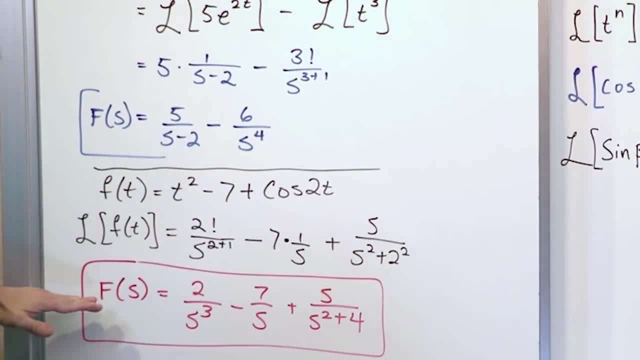 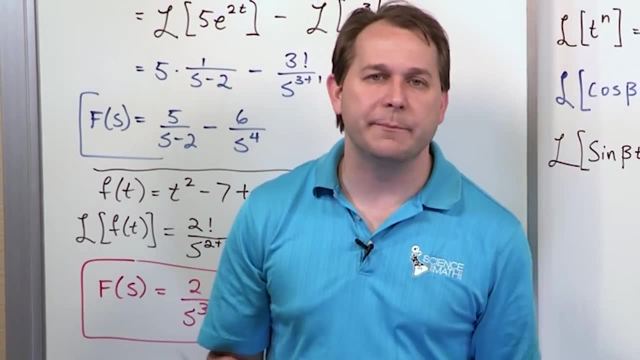 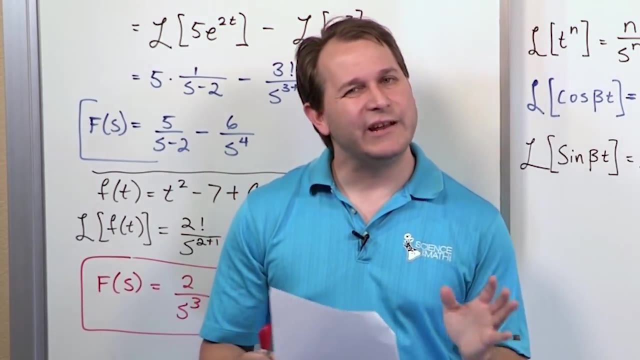 again, this is a pure function of time we have transformed into a pure function of s. if you end up with the Laplace transform, that has anything other than just s's and numbers, you've done something wrong. so that's just something you need to think about. what we've done in this lesson is we're just inching our